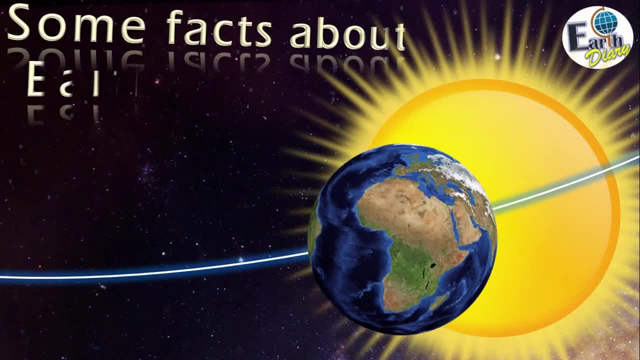 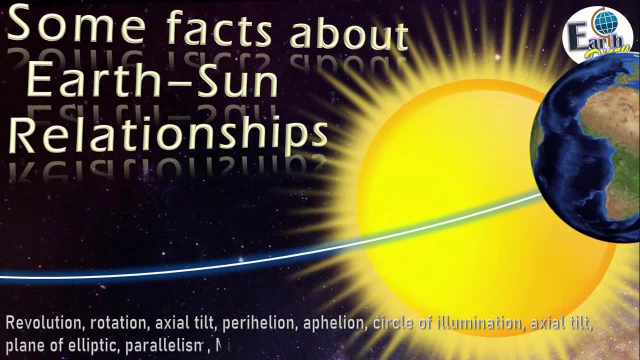 In this video, we will review some facts about Earth-Sun relationships like revolution, rotation, axial tilt, perihelion, aphelion, circle of illumination, plane of elliptic parallelism, Milankovitch cycles, eccentricities, obliquity and precession. 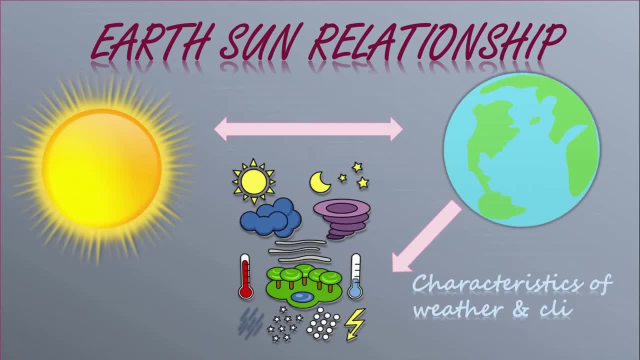 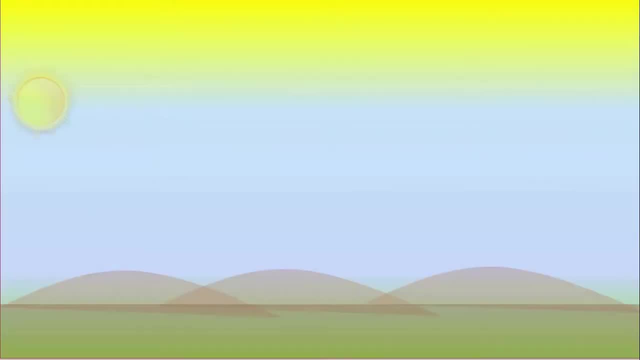 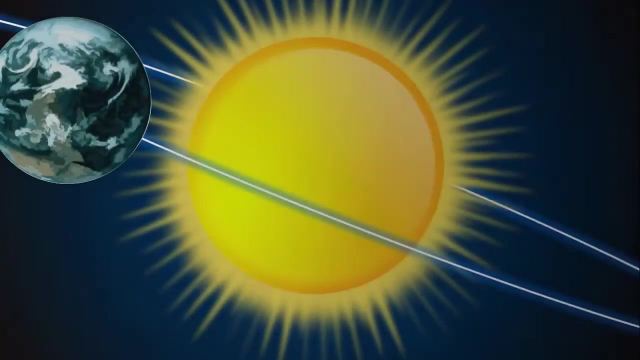 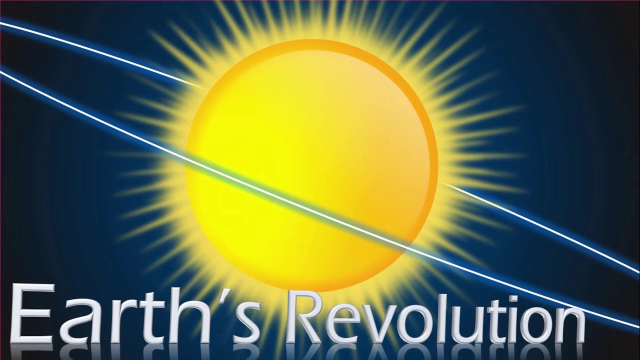 Earth-Sun relationships are important as they help us to understand the characteristics of climate on Earth. They are in charge for daily and seasonal cycles of energy and temperature. Let us review the process of revolution of Earth around the Sun. The Earth complete one orbit around the Sun in about 365 days. 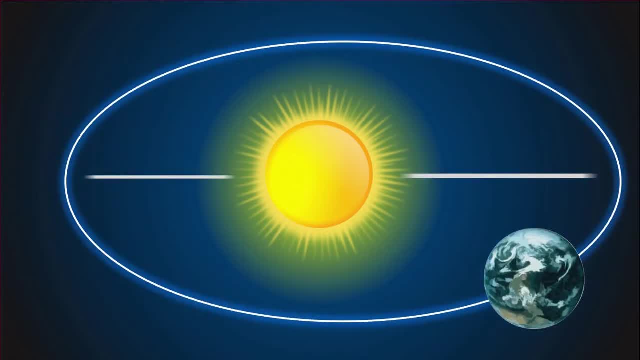 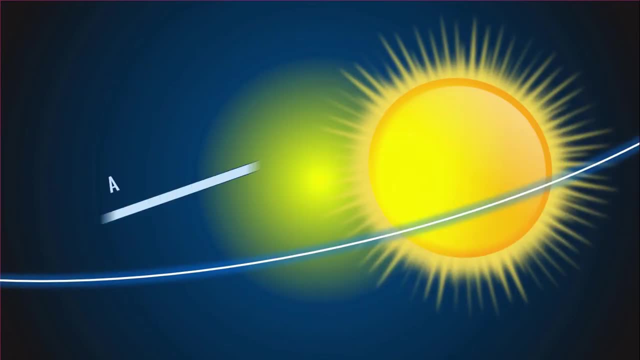 Earth's orbit around the Sun is not circular but elliptical, And Sun is not in the center of the Earth's elliptical path. The average distance from Earth to the Sun throughout the year is 149.5 km, Or 92.96 million miles. 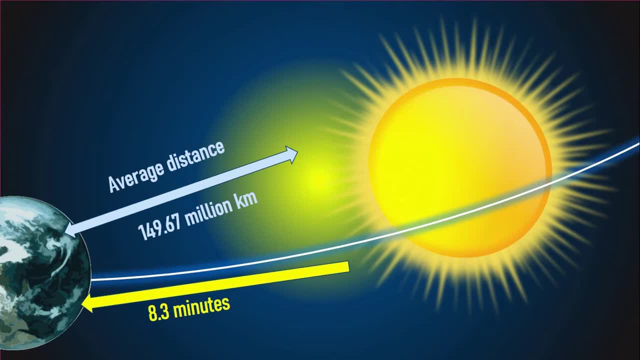 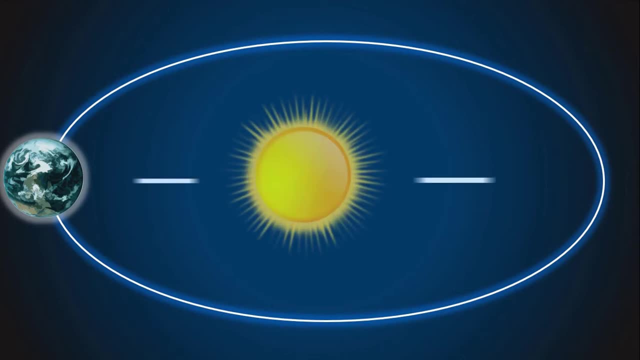 Considering speed of light, it takes approximately 8.3 minutes for Sun's rays to reach Earth's atmosphere. As discussed earlier, the Earth-Sun distance is not same throughout the year On and around January 3rd it is approximately 147.09 million km, which is termed as perihelion, or when Sun and Earth are nearest. And on July 4th, the distance between Earth and Sun is approximately 147.09 million km, Or when Sun and Earth are nearest, And on July 4th, the distance between Earth and Sun is approximately 147.09 million km. 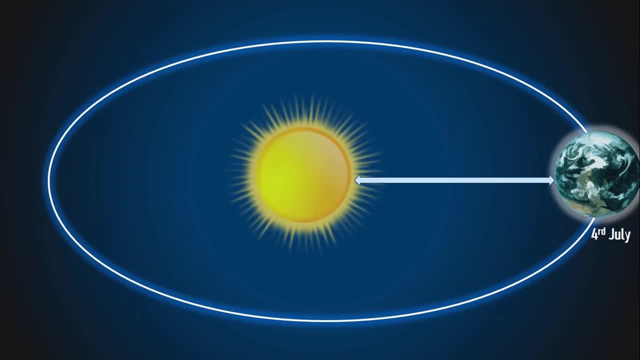 Or when Sun and Earth are nearest- The Earth-Sun distance is maximum, which is about 151.92 million km, termed as aphelion- or when Sun and Earth are the farthest. Rotation is the spin of the Earth on its axis. 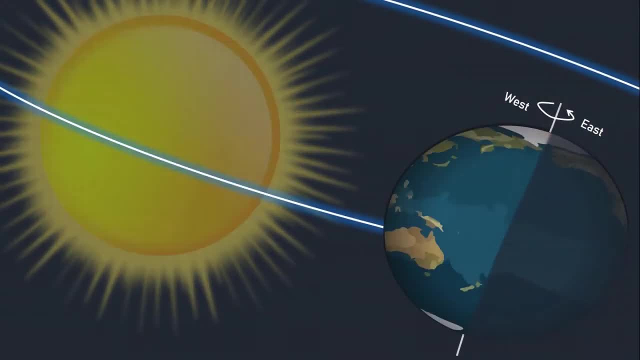 The direction of rotation is from west to east or counterclockwise. when viewed from above, the North Pole. Exactly one half of Earth is illuminated by Sun at any given time. The circle of illumination is the line which separates the illuminated and dark halves of Earth. 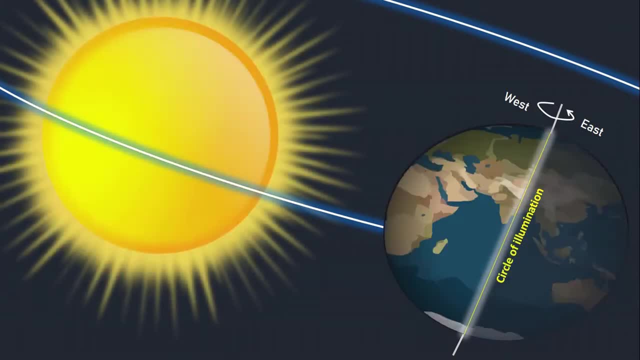 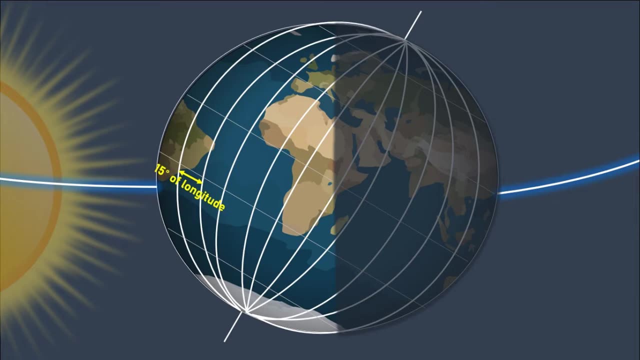 It is constantly changing in position across Earth's surface. One complete rotation of the Earth is completed in every 24 hours. It means that in one hour 15 degrees of longitude is covered. This is also the basis for dividing the Earth into time zones. 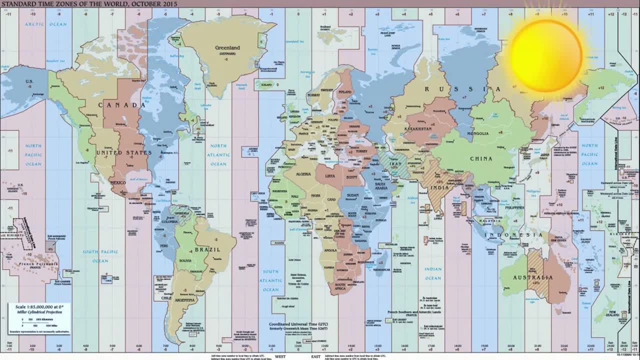 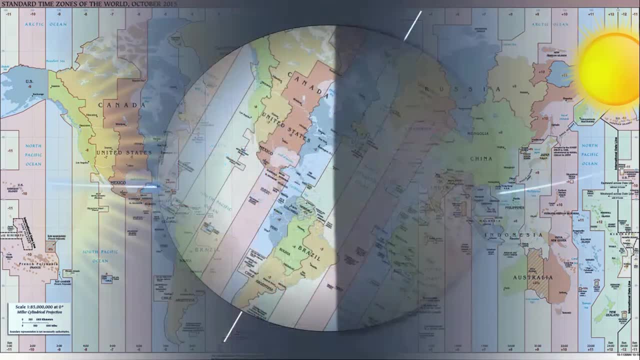 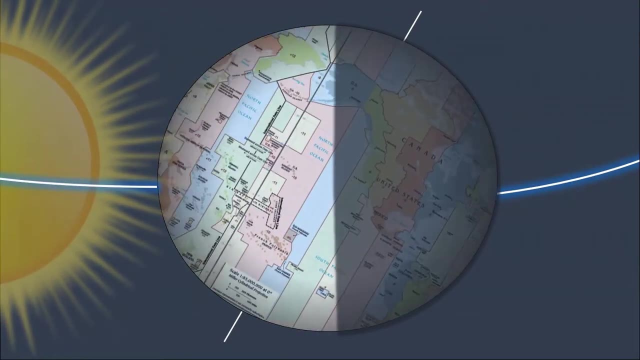 Time zones are 24 longitudinally based regions across the Earth's surface. They are approximately 15 degrees of longitude in width, So every hour one time zone is receiving the direct rays of Sun, and some are on the edge of the illuminated part of Earth, while some are in darkness. 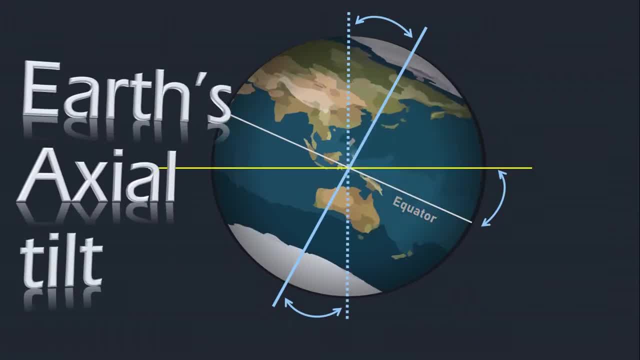 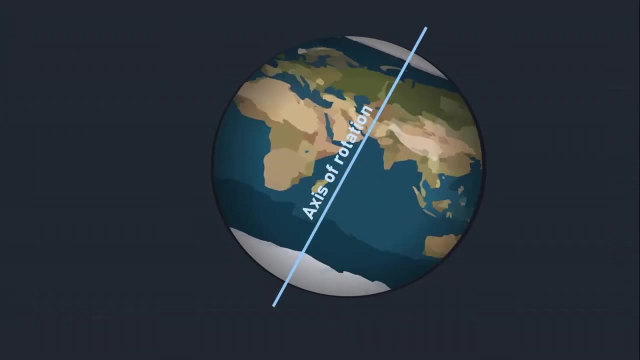 Now let us review Earth's axial tilt and concept of parallelism. The Earth's axis is not vertically straight but tilted. In fact, all the planets of our solar system except a few have tilted vertically axis. the Earth's axis of rotation passes through both poles and has a tilt angle of 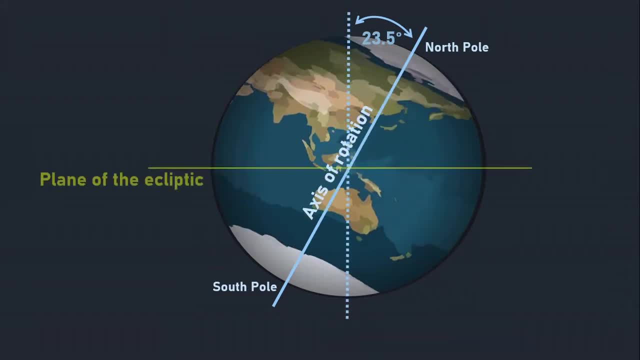 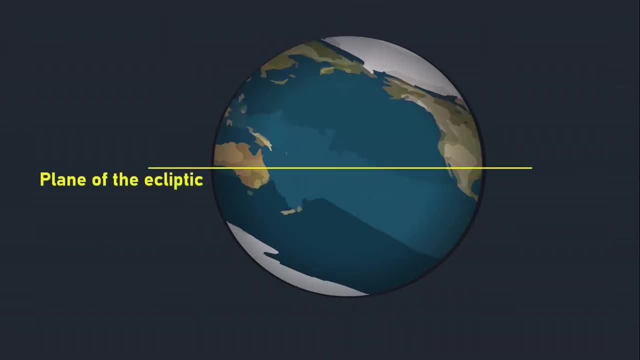 23.5 degrees. This tilt is calculated from the perpendicular line through the plane of the ecliptic. The plane of the ecliptic is the imaginary horizontal plane on which Earth revolves around the Sun. Now, if a perpendicular line is drawn through Earth and the plane of the ecliptic, 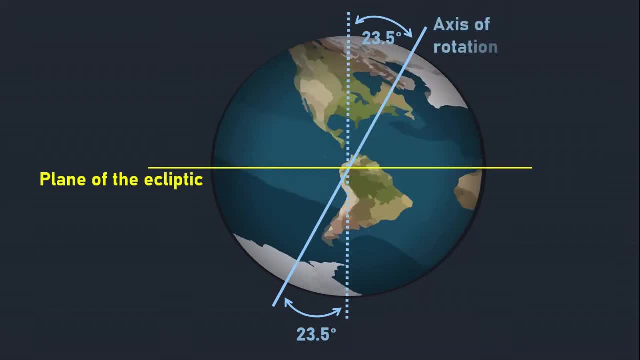 The axis of rotation lies 23.5 degrees from the perpendicular line and the plane of the ecliptic. Likewise, the equator is also tilted 23.5 degrees from the plane of the ecliptic. This 23.5 degrees axial tilt is almost fixed. 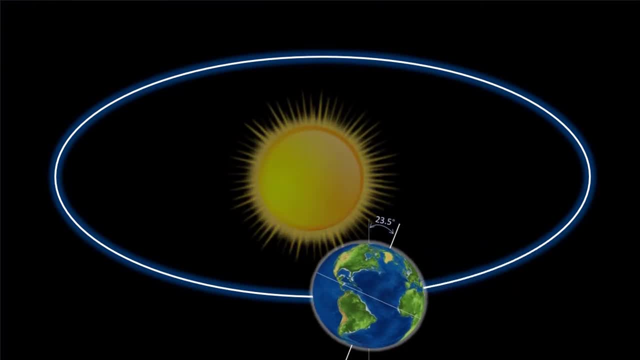 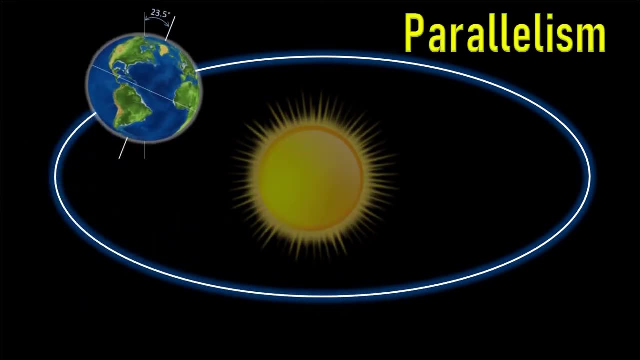 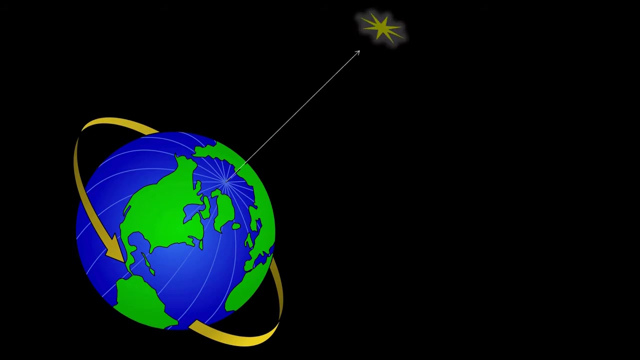 No matter where Earth is positioned in its revolution around the Sun, the axis points in the same direction and remains at the same angle. This principle is known as parallelism. The Earth's axis of rotation has a reference point in space, which is Polaris or the North. 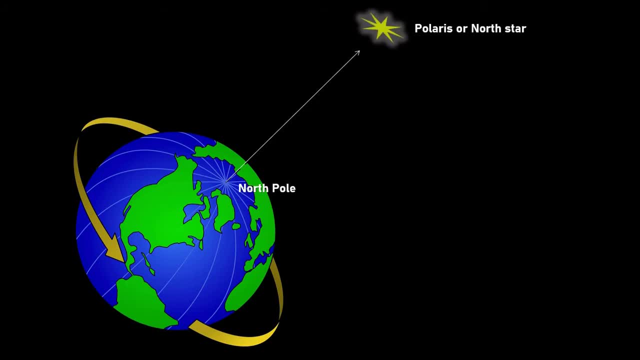 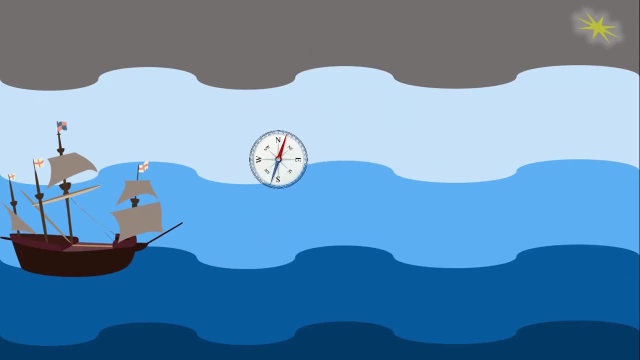 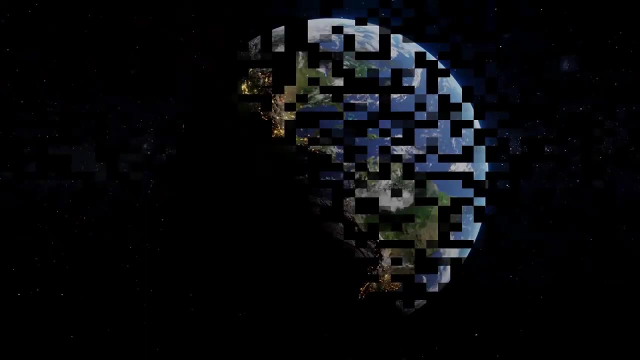 Star, The North Pole of the Earth always points towards the Polaris. In old times, this knowledge was used by sailors for navigation purposes. However, scientists have not been able to prove this. However, scientists have not been able to prove this. 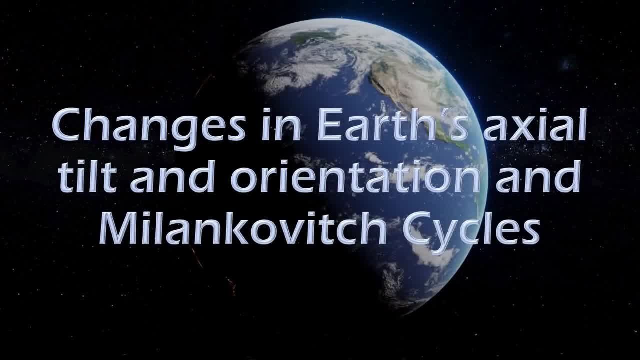 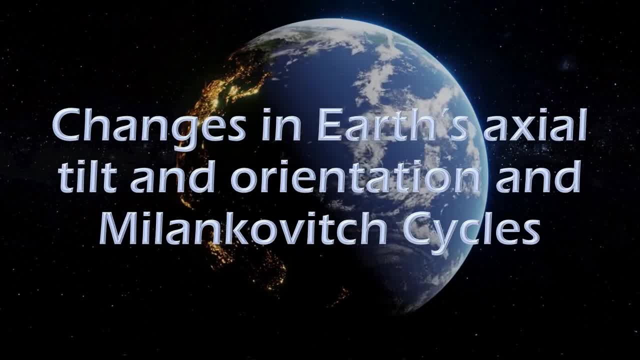 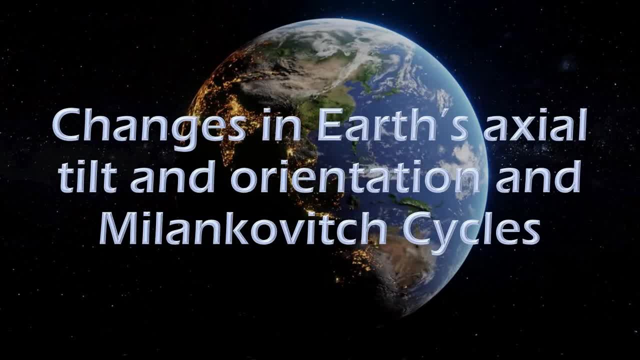 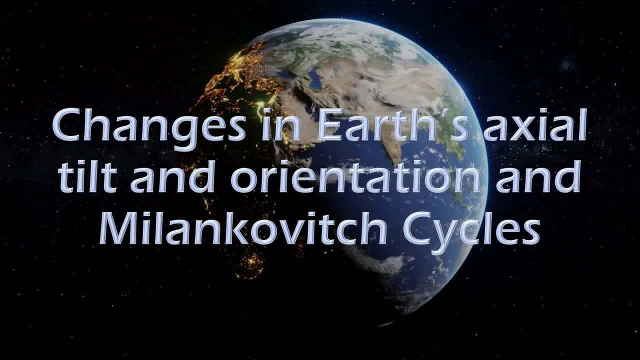 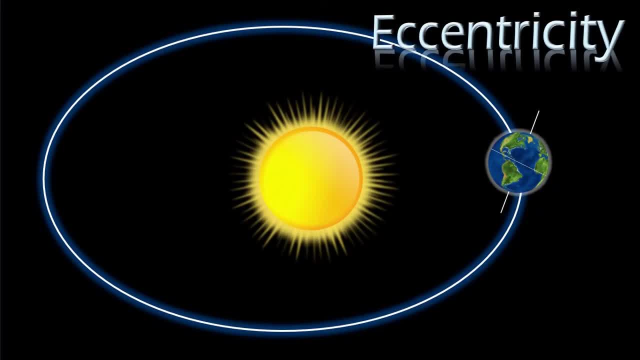 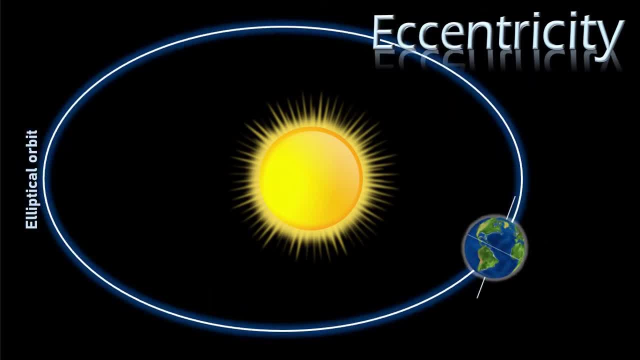 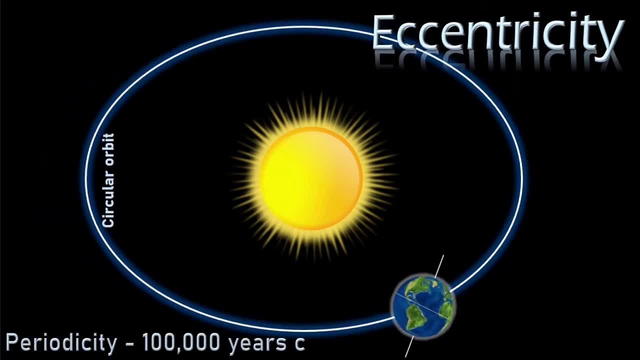 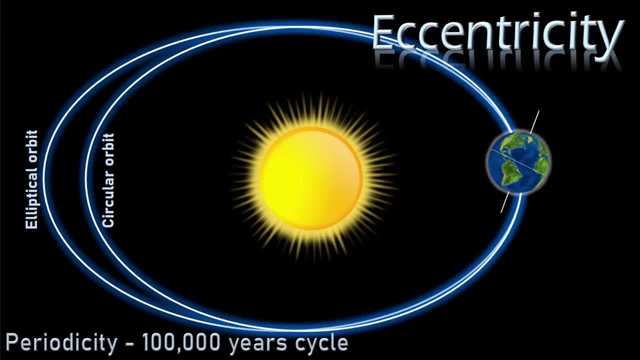 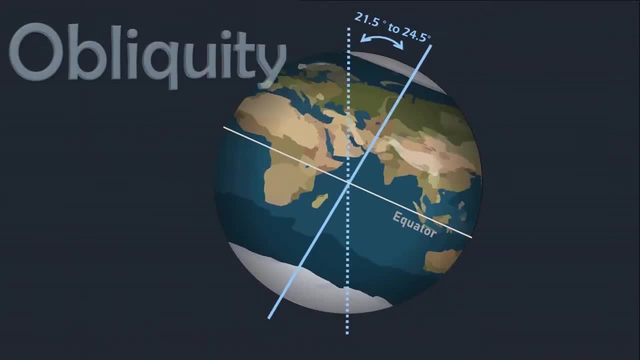 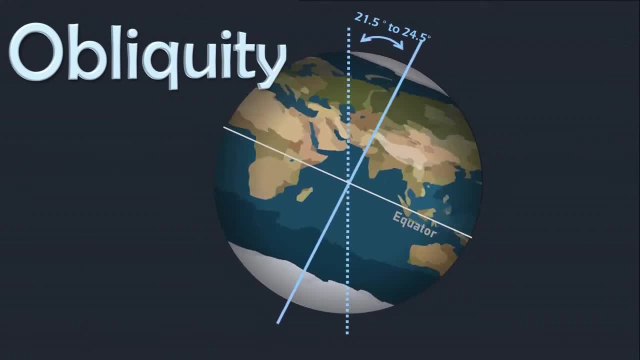 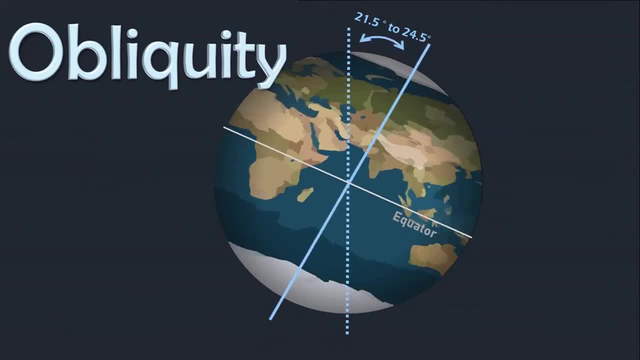 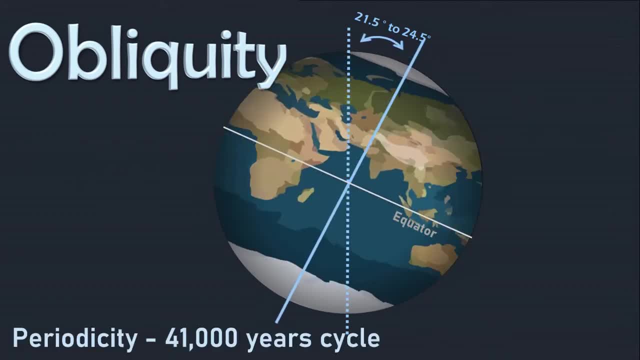 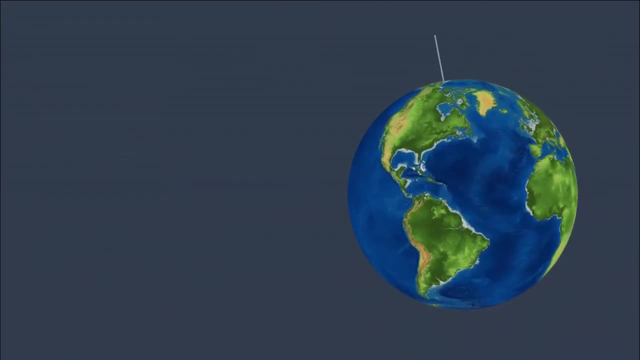 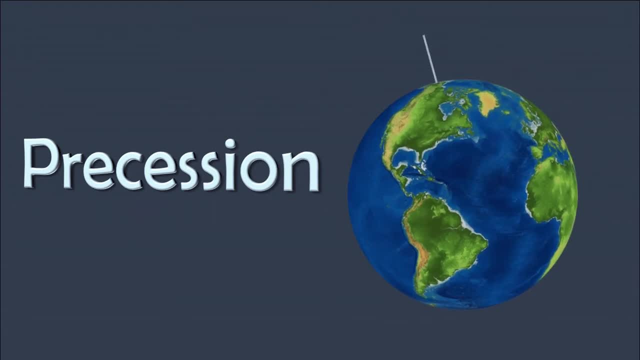 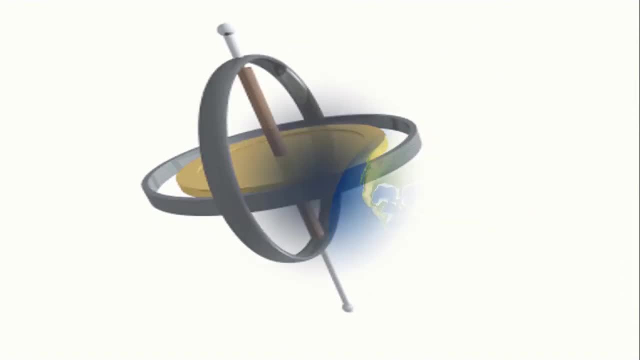 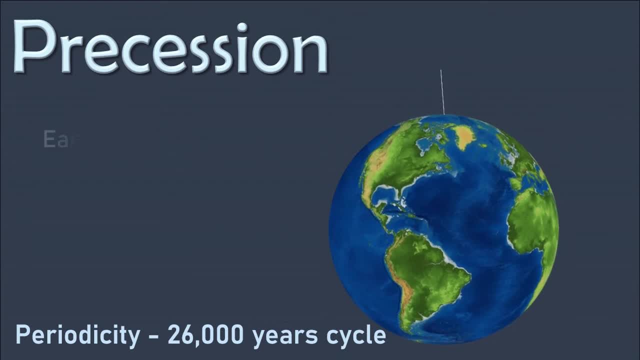 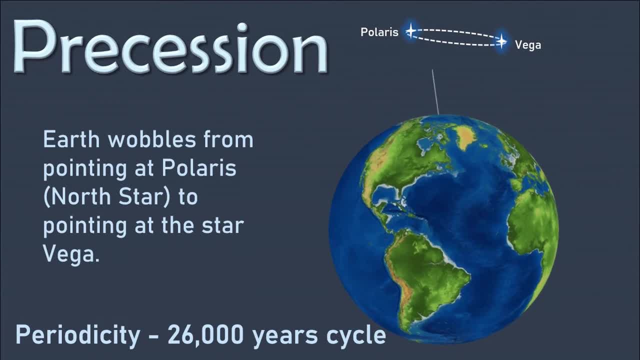 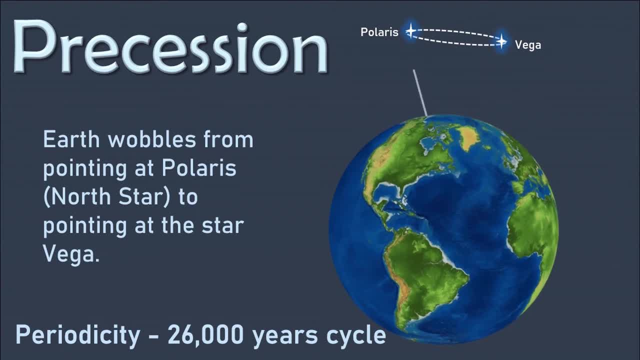 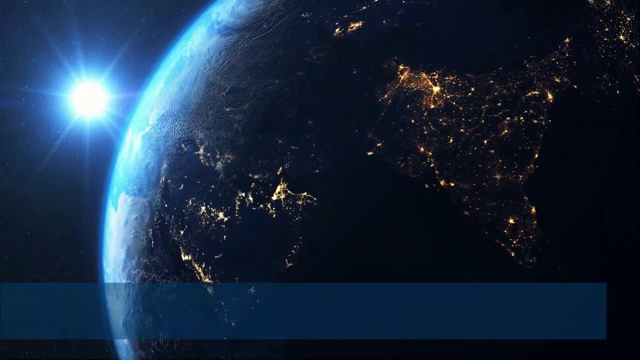 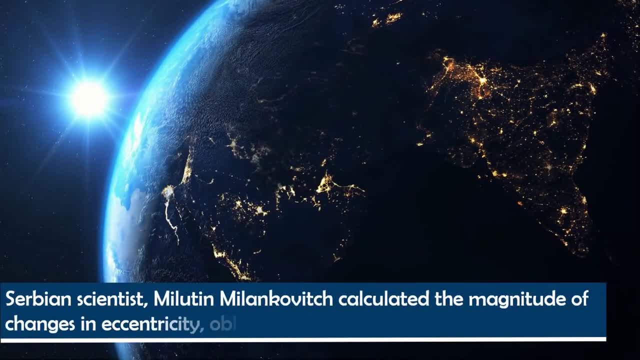 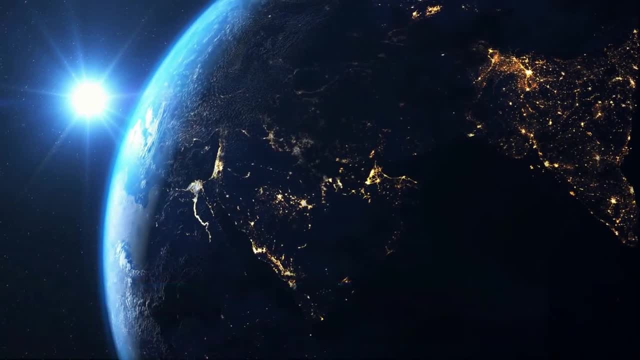